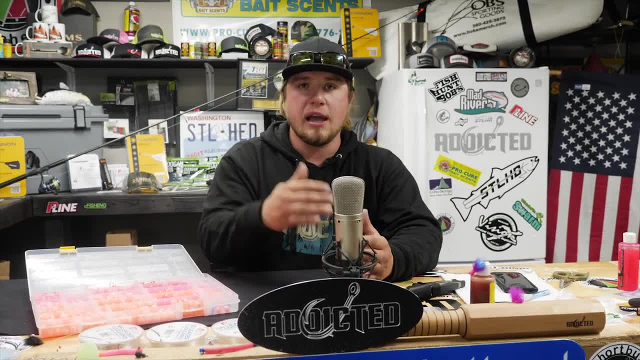 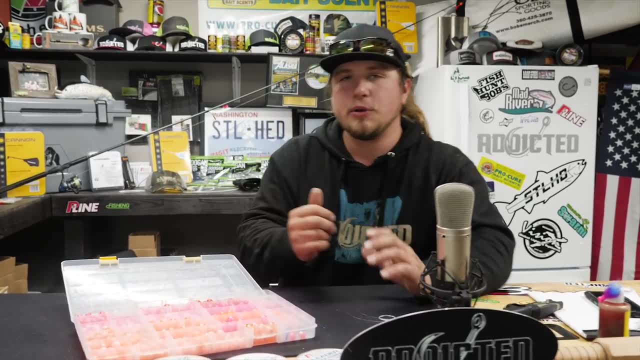 where to start and then things that you could do to progress your bead fishing and move a little bit farther in colors and sizes. so first things first. we're gonna start here, looking at our box, what I'm gonna do every day I go to the river, or if I'm in the tackle shop looking I want to have a. 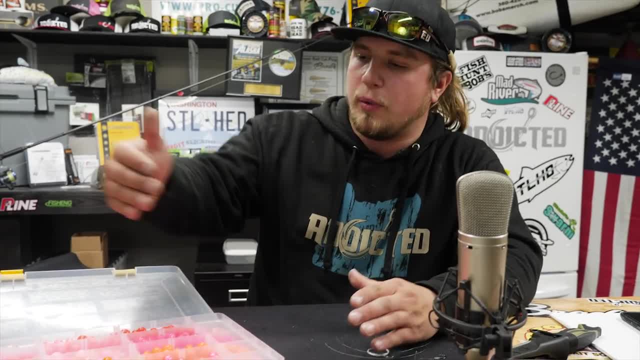 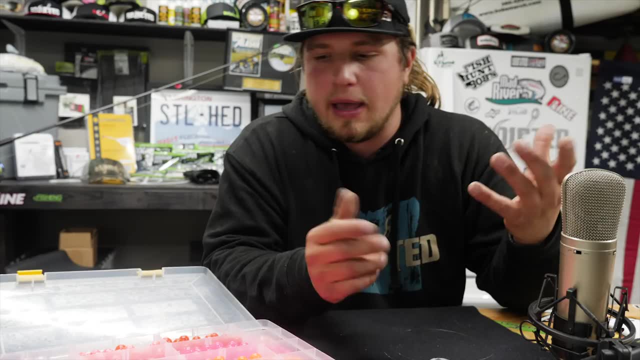 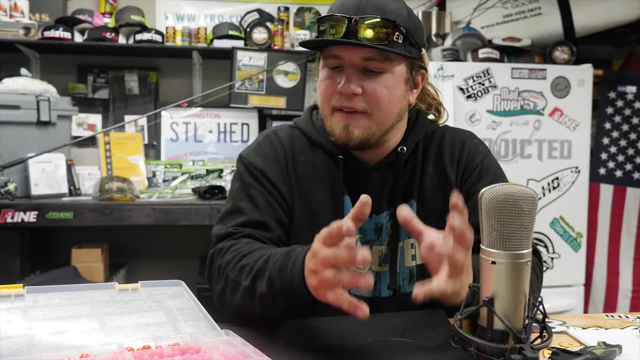 good range of colors. range of colors I mean from pink all the way to hot orange, even red. so pink, orange and red are gonna be your main contrast of egg colors or natural colors that go down the river. we have a peach color here as well, more of a dead egg, a natural color here, but having three 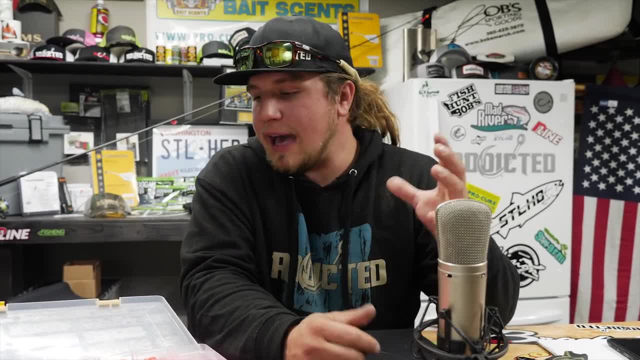 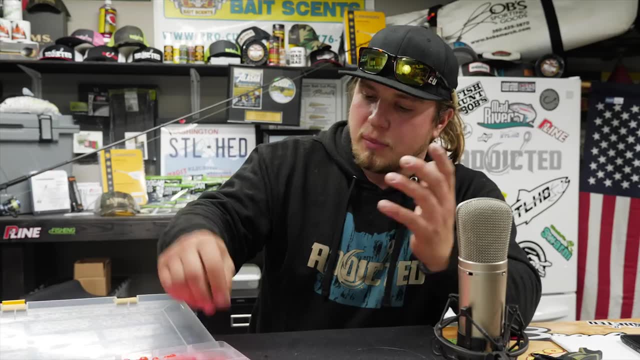 styles of beads is. I would say it would be crucial having different presentations that you can use in a hole or on a double set up so that the fish constantly has a different choice. my pink beads. I usually always like to fish on a clear day. if I have blue sky or any kind of clear weather. I 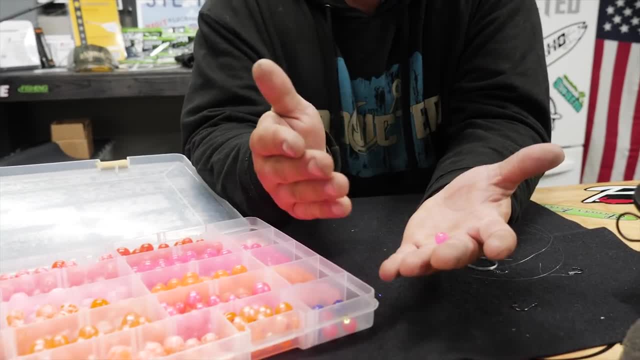 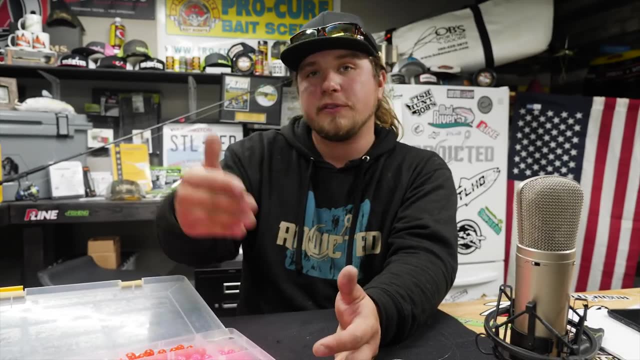 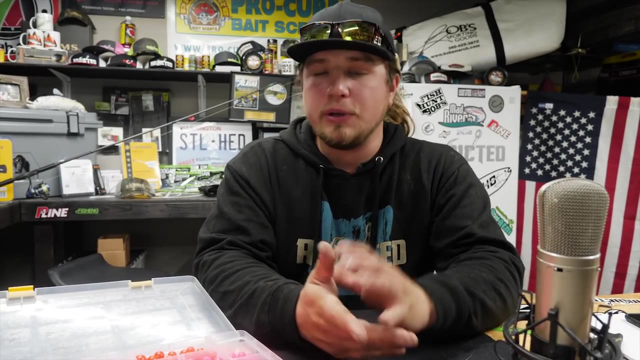 usually range more towards pink, so sizes are very important. having a good range of size of beads in your box is probably the most important part of it. eights, tens, 12s, 14, sometimes even up to 16 millimeter beads can be extremely effective. the key is to have them in your box. you don't need a. 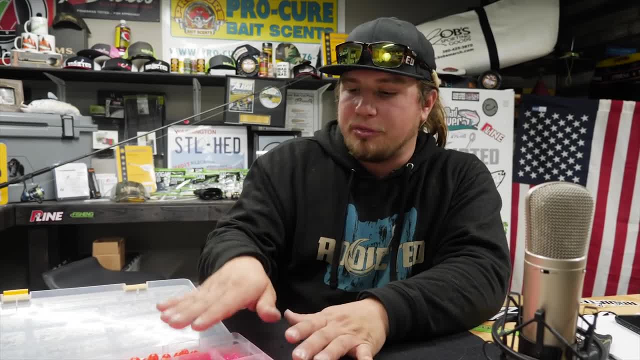 lot of each color, but just make sure that you have them in your box. you don't need a lot of each color, but just make sure that you have them in your box. you don't need a lot of each color, but just try to have each of your favorite colors. have three sizes of pink. have three sizes of orange. 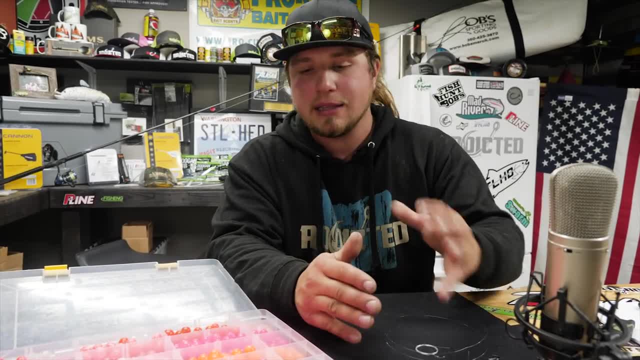 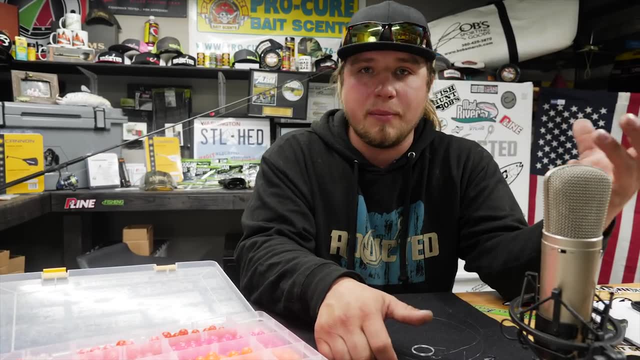 and have three sizes of red, because there may be one day out there on the river that only one size of egg is gonna work, having an egg that is a different or a bead that is a different, attractor to a different time and the spawning can be very important as well. so having three different sizes, 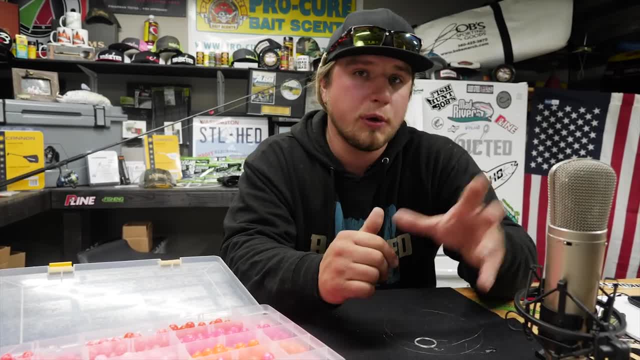 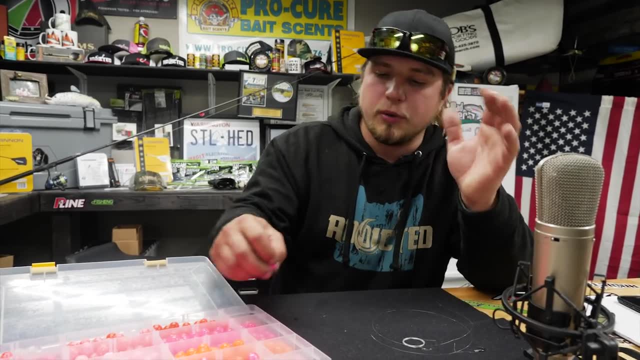 having three different colors is crucial. don't go in there and blow your money on all the same style of bead. be sure to have that range and that variation of color and size. so what I would start with always if I'm gonna go up to the river and it's a clear day, is a pink color. 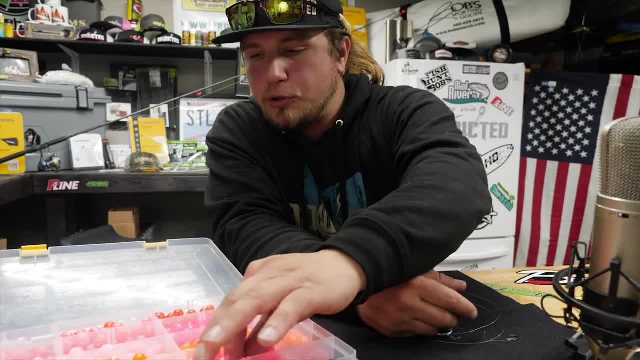 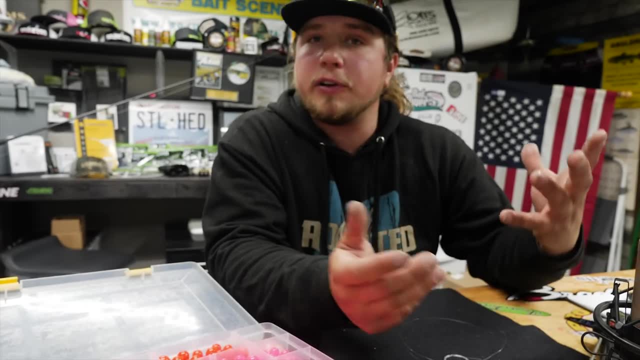 whether it be a pink that has some sort of a blue hue to it, a light pink with more of a frosty look on it, and if the water is clear, I might go towards a smaller bead for a smaller presentation, because clear water actually illuminates these beads too, so that they have the illusion that they're 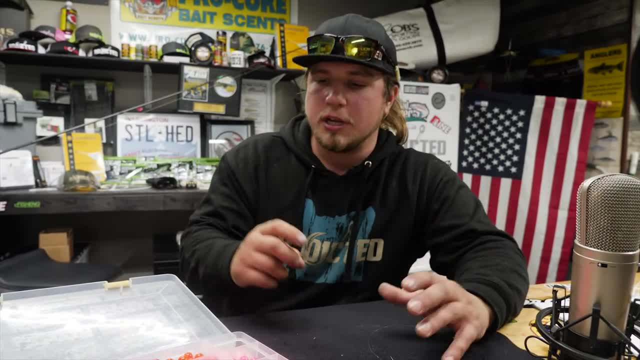 actually bigger than they are when they're in the water and in front of the fish. what I like to do is start small and work my way up. the key is, especially if you have, or are allowed to have, a double set-up and a double set-up, you just have to have a double set-up. you just have to have a. 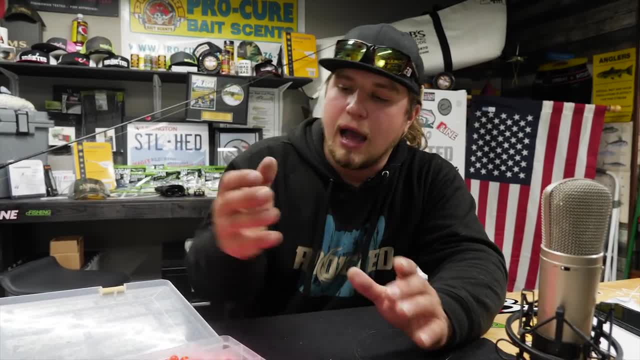 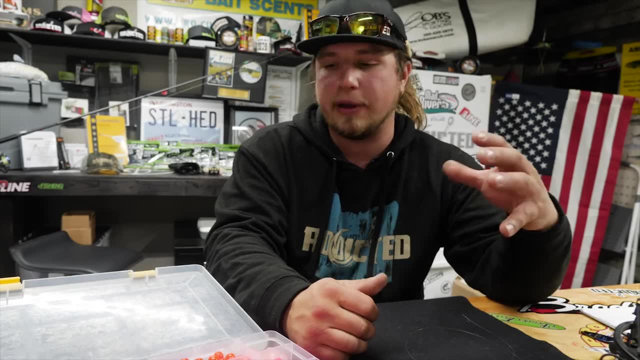 on your river is fishing two different size beads. in my opinion, I might start with a 14 mil on my top hook and put a 12 or a 10 mil on my bottom hook, so that I'm covering that size range. One thing I also like to do is use two different 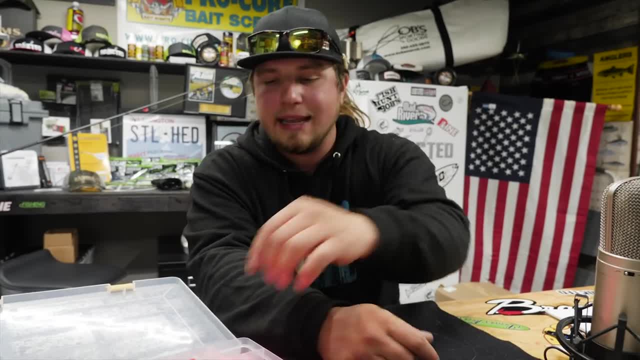 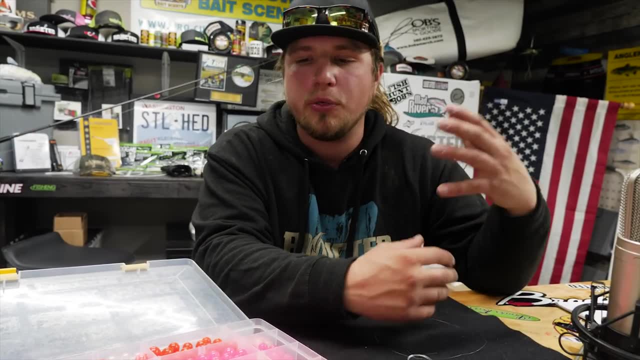 colors of beads at the same time, if possible. If not, I take this soft bead off, I change it to the different color and I keep fishing in the hole And you'll notice time and time again as you change and go through that variation of 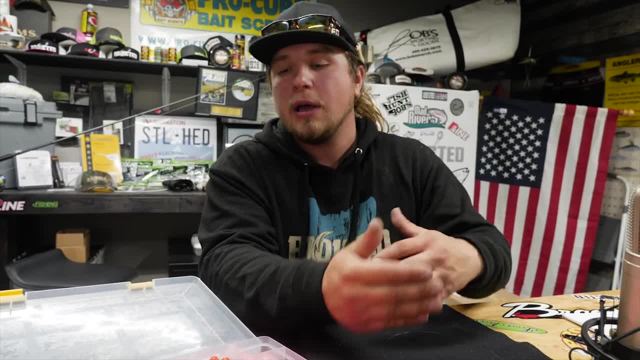 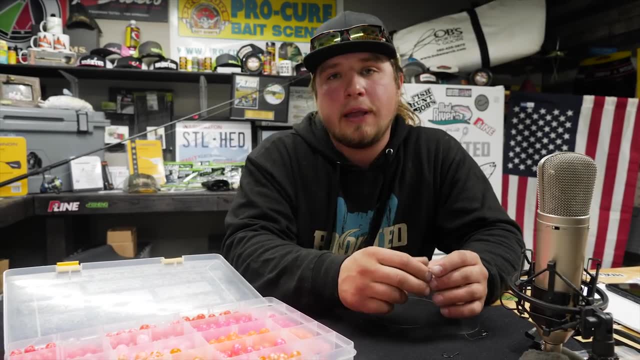 beads that you'll find success immediately after changing. So you're having that range, having three different sizes, having three different colors, and using each of them in a hole will up your game and allow you to catch a lot more fish on these beads. So the second most important part of using 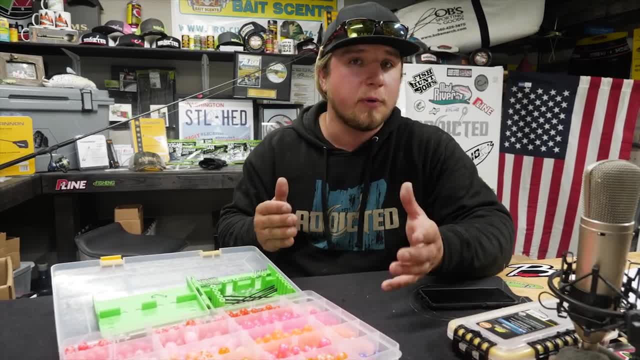 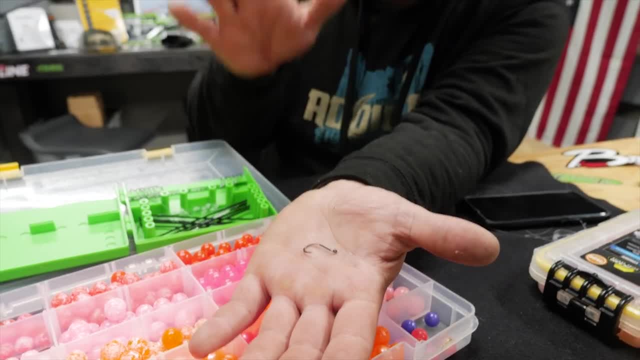 these beads is going to be your hook choice. What I like to use is a number four size hook. We have one right here. These are some beautiful must-add hooks that we have. Number four, and I never really go above a size two hook, The. 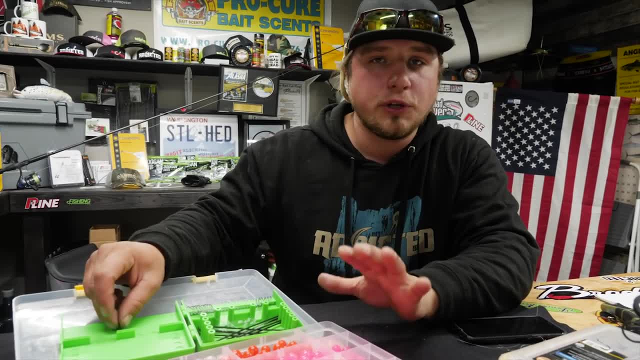 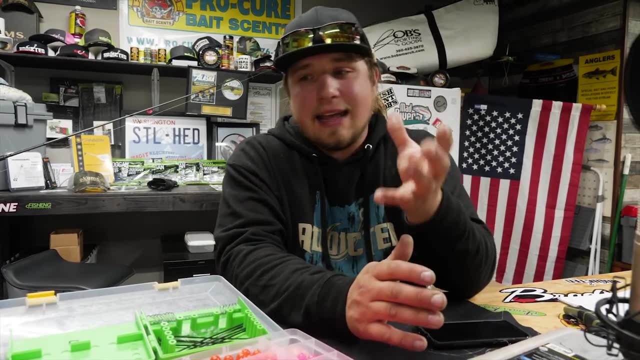 times that I will go to a size two hook is if I'm going to use 14 mil beads, and that's about the only time If I'm fishing anything smaller than a 12 mil, 6,, 8,, 10s, up to 12s- I'm going to use a number four. hook so that that hook doesn't actually weigh down my presentation and drag that bead towards the bottom When you have a number 14 or a 14 mil bead. why you want a size two hook is so that when that bead, if it accidentally does, 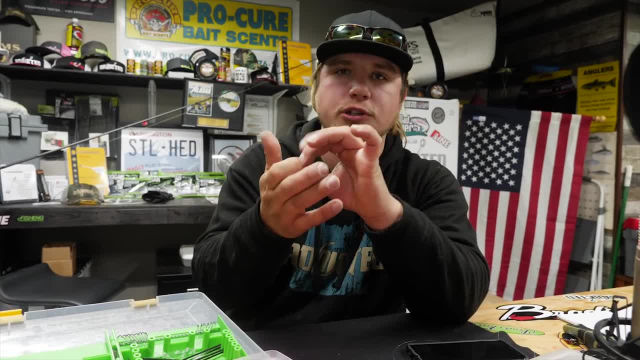 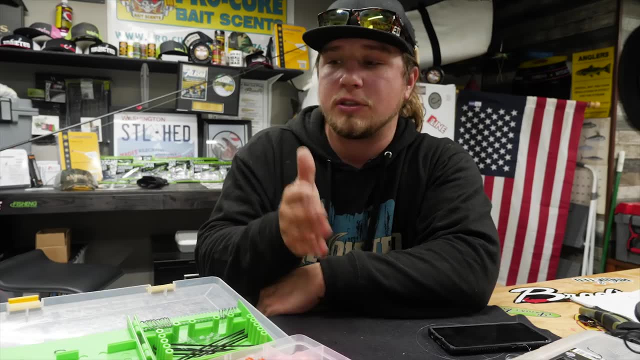 slide down to that hook, you have a bigger hook gap and actually a larger hook that will withstand the pressure of that bead sliding down onto that hook. Number four hooks- number two hooks- are key for this style of fishing. Be sure to have both of them in your pack if you're going to be fishing anything over a 14 mil. 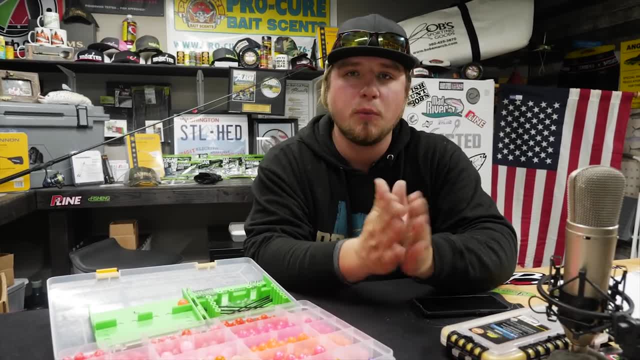 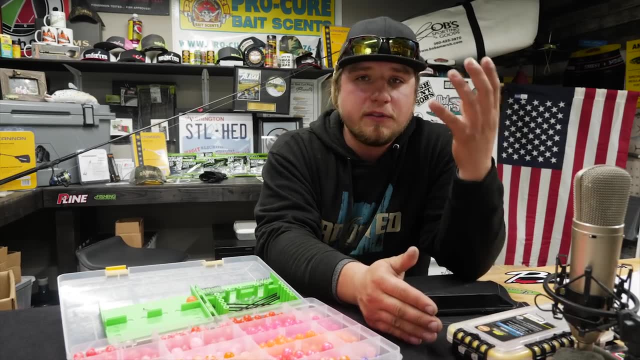 bead. Thanks for tuning in everybody. If you guys have any questions or you want to learn more about the logistics of these beads, be sure to comment below and ask some questions so that we can figure out what you guys want to see, what you want to learn and if you can find something that I didn't talk about. 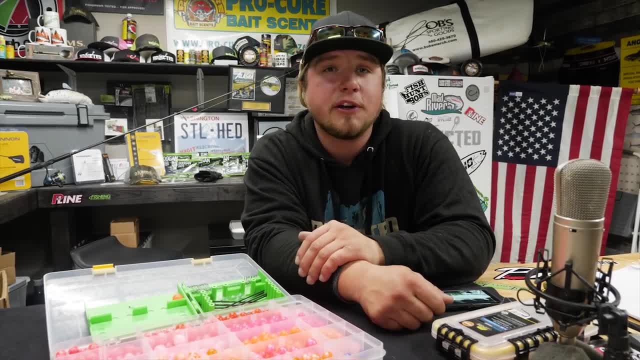 So be sure to comment below, like and share this video out there. subscribe to our YouTube channel, guys, because we have a lot more to share with you guys. I'll see you in the next video. Bye, If you have how-to's coming out every day, that'll make you guys a better.